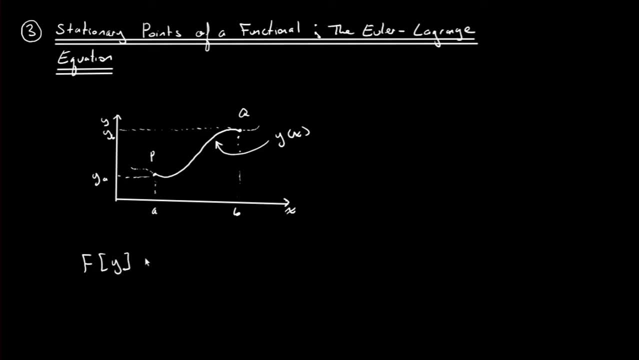 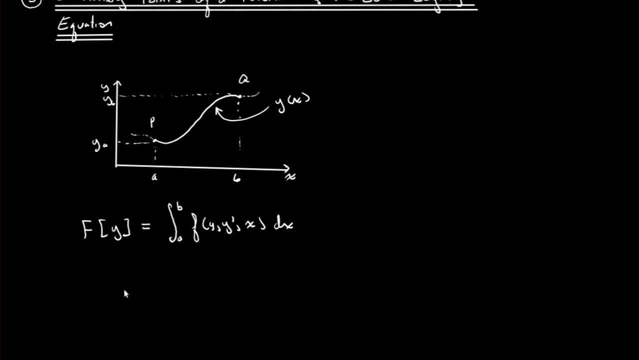 of a functional f of y and that's got to be equal to the integral from a to b of some function of y, y prime, and it might have some explicit dependence on x and integrate with respect to x. that's the definite integral and what this does is it takes a function y and it maps it onto. 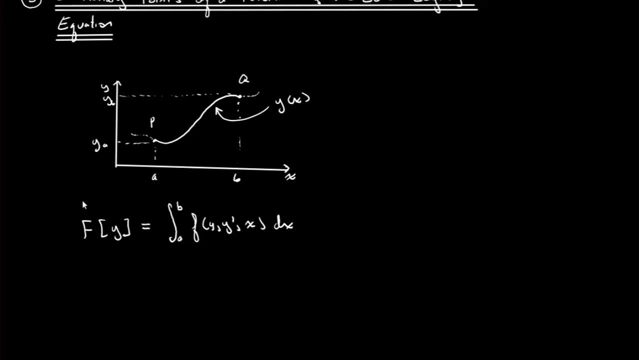 a scalar f of y, and the problem is, the problem is to find stationary points, or we should put that in quotation marks: stationary points y of x, of the functional f of y. okay, and we're going to go about this in the same way we went about solving the general 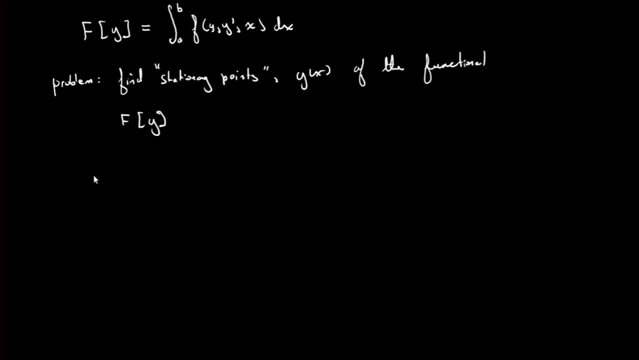 n-dimensional case by starting with our functional and making instead of a small displacement. the language we use in calculus of variations is well, naturally a variation, so we start with y of x and we go to: oops, please excuse me. well, yeah, of course. no, we start with y of x and we go to. 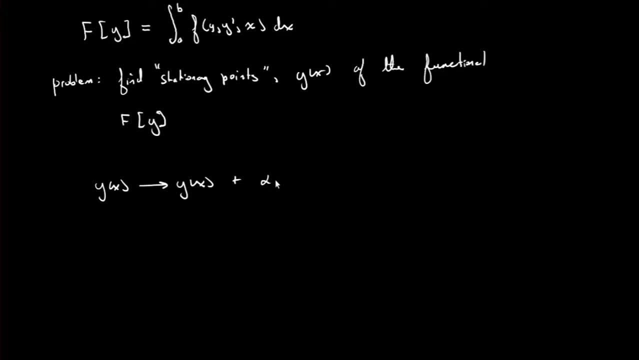 y of x plus alpha eta of x, and it's worth commenting on this because it's a little different to how we did it before. we always had h's as our displacements, but this time i've written it a bit funny. i've written it as alpha eta of x, and it's worth just. 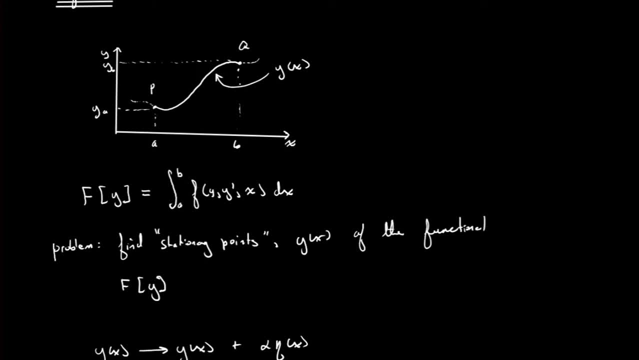 annotating it a little bit. and then we go to alpha eta of x and we go to alpha eta of x and we're going to start by creating this diagram to explain what we mean. so let's say i have function eta of x, like this right and notice i have had eta of x, so i'm going to call this. 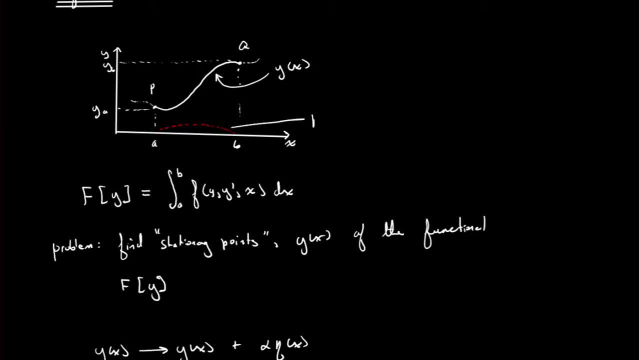 uh, eta plus of x. i've had eta plus of x, um vanish at both a and b, and then, if i do that, i'm going to have eta plus of x. and then if i do that, i'm going to have eta plus of x. and then if i just kind of draw up here what that might look like, uh, what alpha. 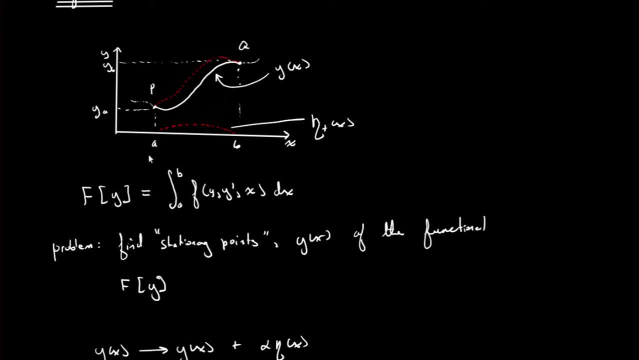 eta of x plus y of x might look like. what i'll get is something like this: so i might call that y of x plus alpha, eta plus of x, and of course, we can have any kind of displacement we like. so our displacement might look like this as well. so it could be negative and i'm going to call this. 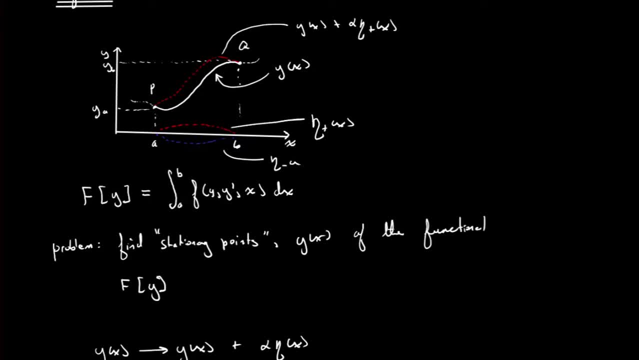 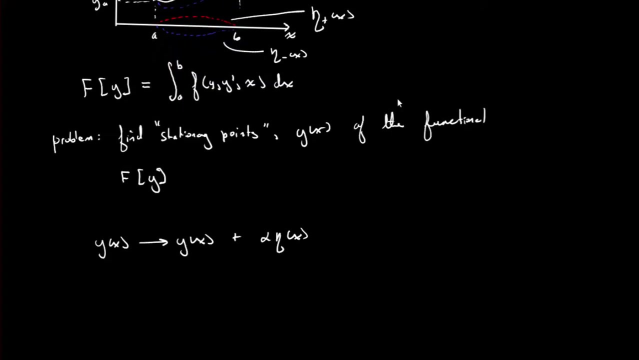 uh eta minus of x, and then we're going to draw in f of x minus. so so this is y of x mark up, sorry, plus alpha eta minus of x. so clearly we are just trying to find all of this. so we're going to draw in alpha eta minus of x and then we're going to draw in. 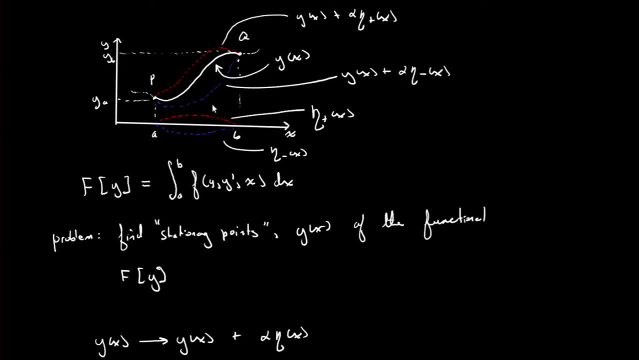 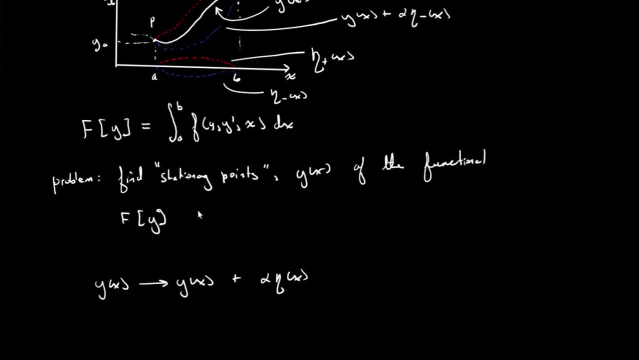 all of the ways to vary the function y. we're trying to find all the ways to vary the function y, uh, so that, uh, the end point stays the same, so that we always land on the points p and q, right. and the way we do that is by imposing the condition that eta of x. oh sorry, of course that's. 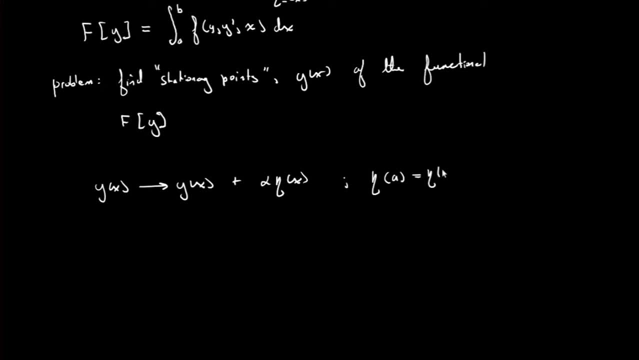 eta of a has got to be equal to eta of b has got to be equal to zero. this is a function, uh, a property that eta must satisfy. and alpha is just small, right, so it's. we can choose it to be arbitrarily small, as small as we would like. so after we make this displacement, 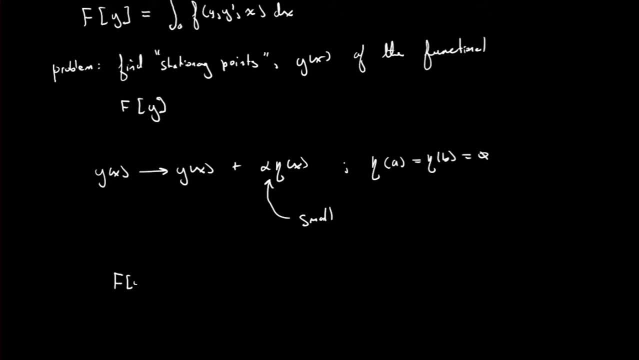 f of y is going to become f of y plus, and this time we use- it's common in calculus of variations to use a lowercase greek delta of f of y to represent the displacement in the value of the functional evaluated at some point that's displaced slightly from the stationary point. okay, now the reason i'm using. 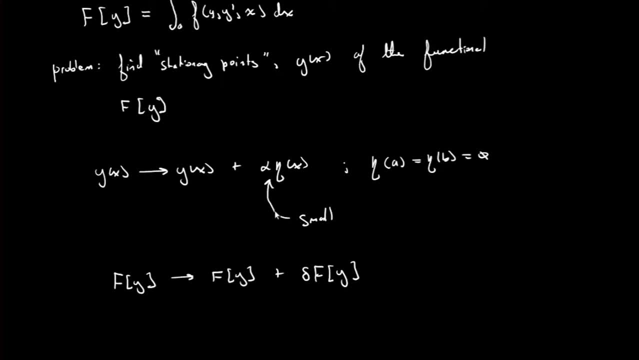 the language of a point is because we can actually think of this as kind of like not just one equation, but it's like an infinite number of equations indexed by the variable f. so this is kind of like uncountably, infinitely many, uh displacements. so it's kind of like 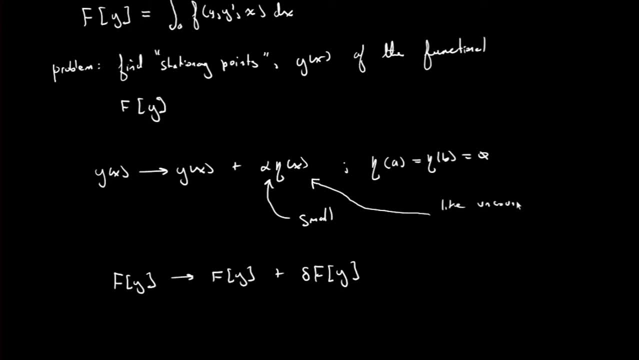 uncountably infinite, infinitely many displacements. so really it's like we're solving the problem in calculus of variations is kind of like taking our work with functions to their logical limit. we started with one variable, we went to n, two variables, we went to arbitrarily many but still finite variables, and now we're 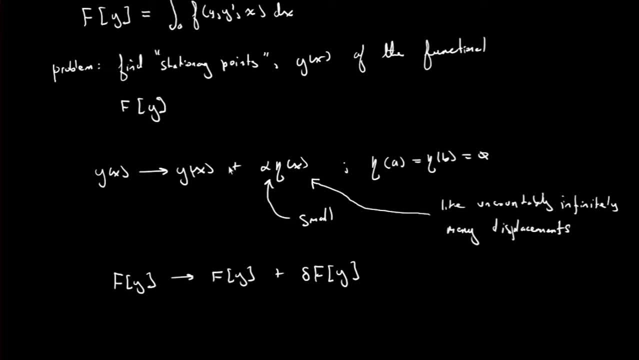 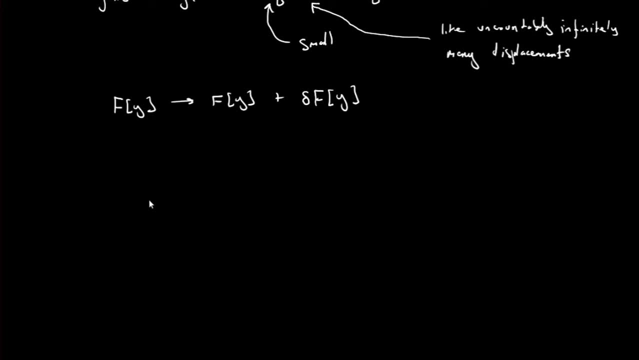 going to uncountably, infinitely many variables. so really, we're going to place the noninter gegnd conditions in the medial units. we're seemed to箕 to play the same game we played before, but just with functionals. We are going to investigate this delta y and we're going to just be bold and we are going to say that delta f of y. 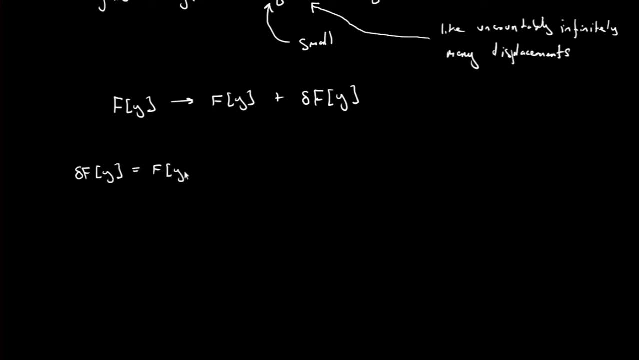 we're going to call that f of y plus alpha, eta minus f of y vanishes to first order in our small parameter alpha, and we are going to say this is equivalent to y being a stationary point Of the functional capital F of y. So now we're going to start our investigation, just like 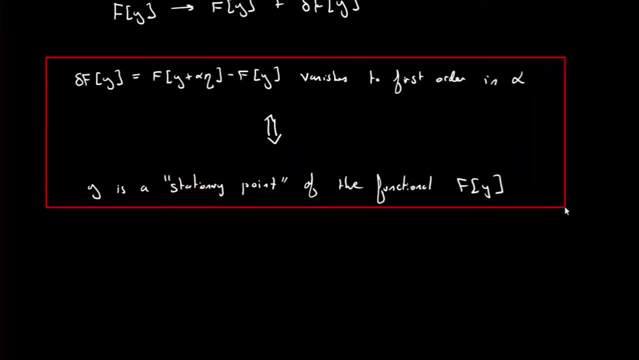 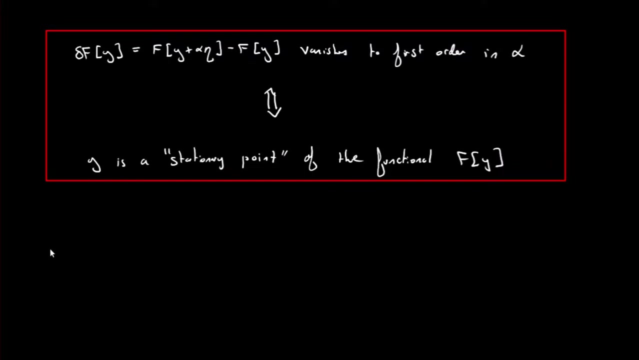 we did before, but we're going to box this off as our definition and then we're going to now investigate our variation In y. that's a consequence of our- sorry, our- variation in f. that is a result of our variation in y. Well, we're just going to start by studying f. we're going to start by studying f of y. 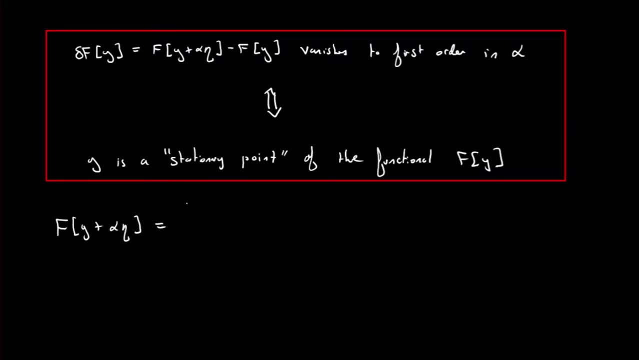 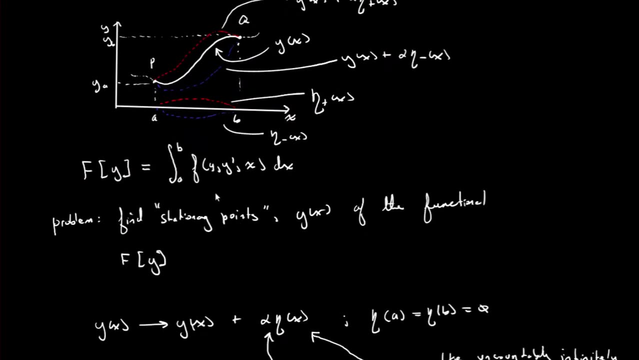 plus alpha eta, and this is clearly just going to be the integral from a to b of lowercase f and looking at our definition up here, Y is just going to become y minus f of y. So we're going to start by studying f of y. 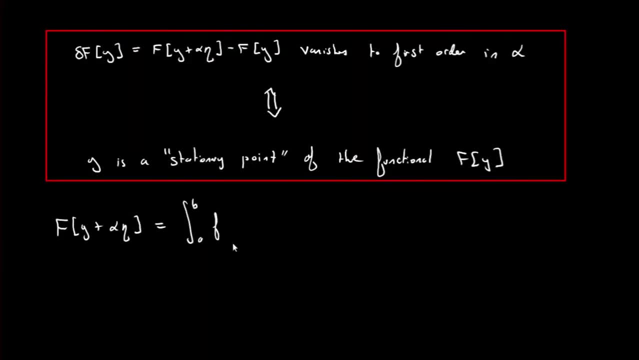 plus alpha eta, and this is clearly just going to be the integral from a to b of lowercase f of y plus eta. So that's going to become f of y plus eta and y prime is going to become- oops, sorry, please excuse me, that's plus alpha eta. 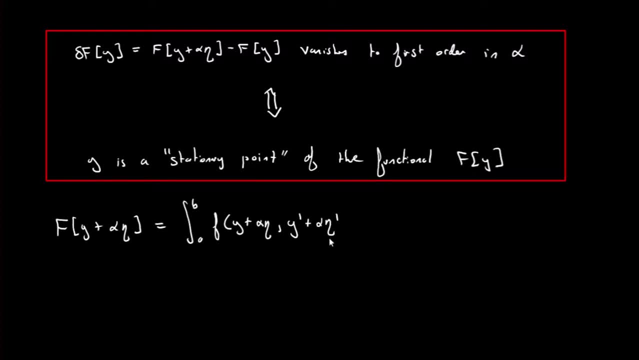 Y prime is going to become y prime plus alpha, eta prime. Remember, alpha is a constant here, it doesn't depend on x, it's a displacement that we are allowed to choose and of course, x just stays the same because it's the function that changes. 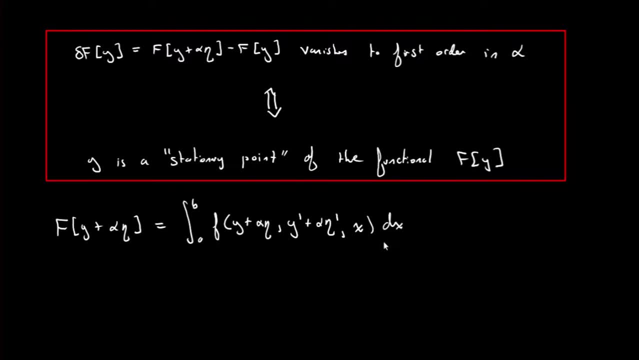 not the point. we choose to evaluate it, and that's evaluated with respect to x. To make any progress, really, we're going to have to do something about that f right, so we can use the tools we used before quite directly to get something useful out of this. 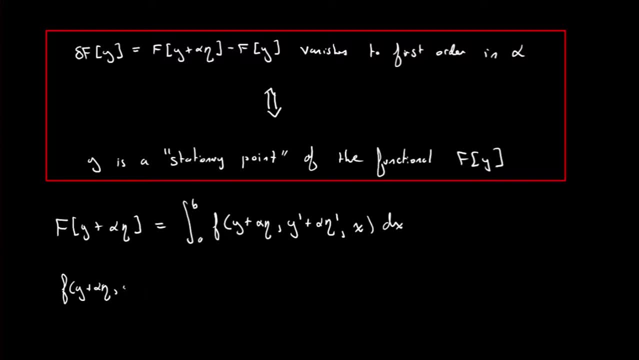 So we write: f of y plus alpha eta is equal to and y prime plus alpha eta prime and x. well, we just use Taylor's theorem. we use Taylor's theorem to expand this and we get f of y, y prime and x. but we also collect plus alpha eta, df dy plus alpha eta prime. 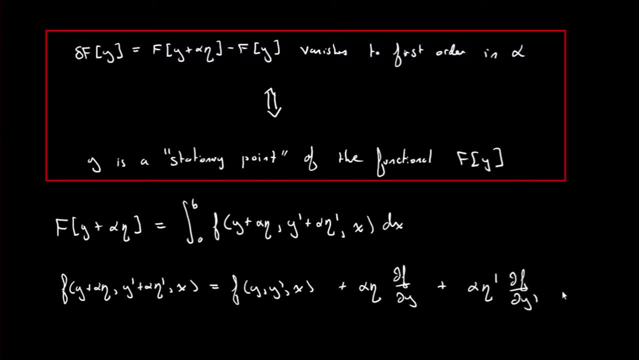 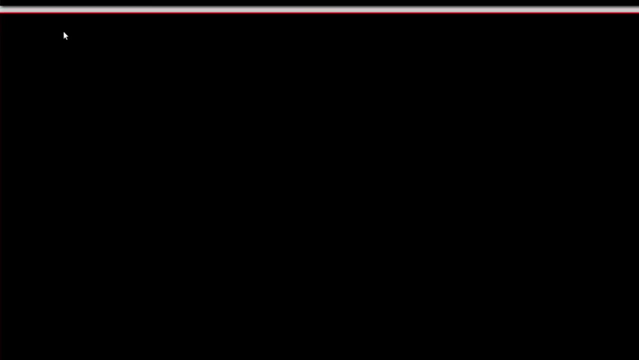 df, dy, prime, Right, Right, Right, Right, Right, Right, And of course, plus higher order terms than alpha squared. so terms of order: alpha squared and higher. Now we are just going to investigate our functional so looking at this, we just stick that under. 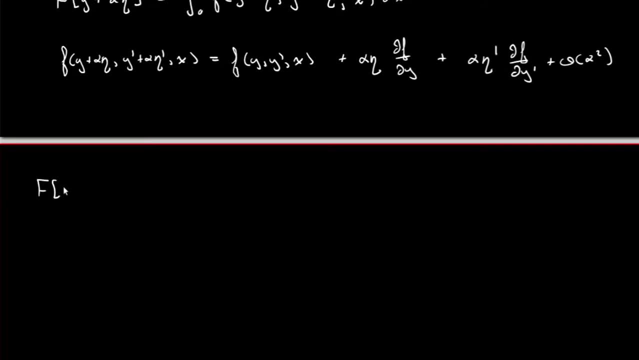 an integral sign to compute our functional of y plus alpha eta is going to be when we stick the right hand side under the integral sign. so we write the integral from a to b to b, of f, of y, y, prime and x, dx and we add in our integral from a to b and we can. 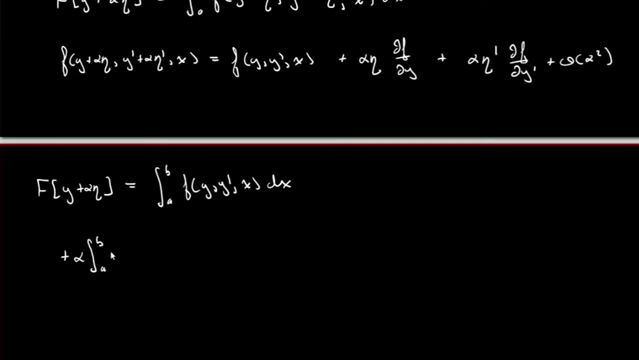 pull the alpha on the outside because, remember, it is a constant, it doesn't depend on x and eta, unfortunately, is a function of x, so it must stay inside of the integral, The partial derivative of f with respect to y and that's integrated with respect to x and 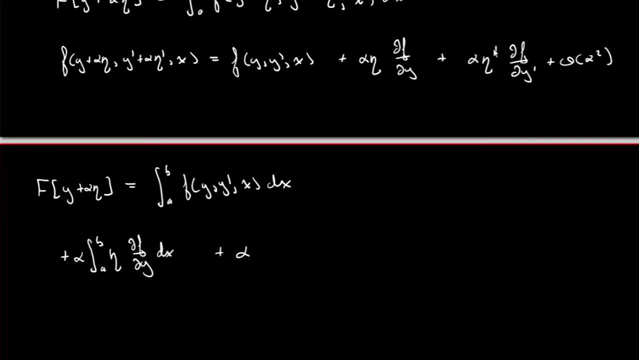 another term, that's alpha. again, that can come out of the integral sign, integral from a to b, and as far as we know, eta prime still depends on x. so we must include that under the integral sign in the most general case and we write partial derivative of f with: 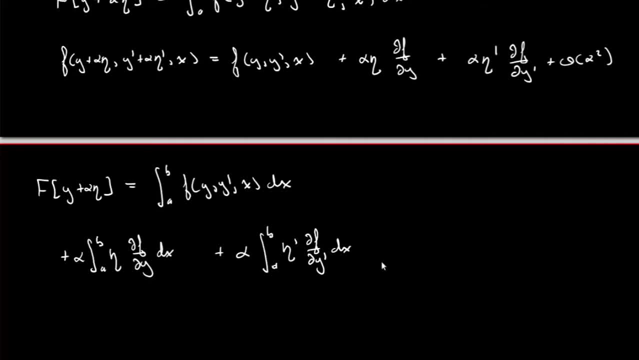 respect to y prime and we integrate that with respect to x and we get the integral of f with respect to x. Of course, we must still keep our terms of higher order than alpha squared, including terms of order alpha squared. Now we recognise this right. This is just our functional evaluated. 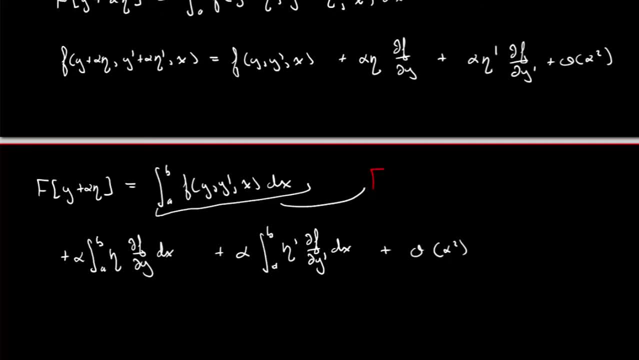 at y. so this here, this here is f of y, This here. we can't really do anything with this, but we would like to simplify this, So we'd like to simplify this, so we're going to give it a name. the name we're going to give it is r. 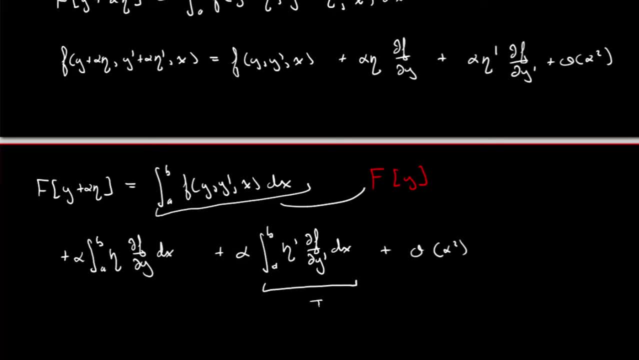 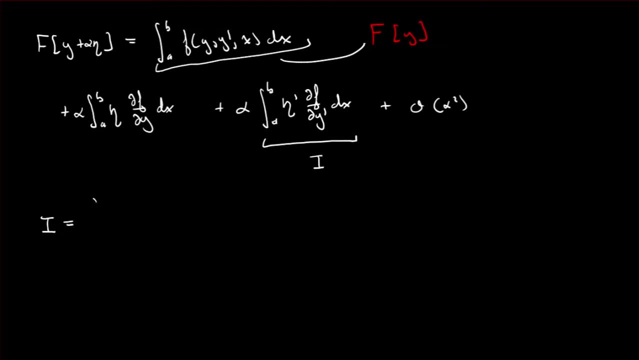 We're going to give it the name i. So we're just going to investigate how we can make i a bit simpler. So we write: i is equal to just the integral from a to b, so excluding alpha, we're just after the integral here. that's eta prime. but instead of writing eta prime, I'm going. 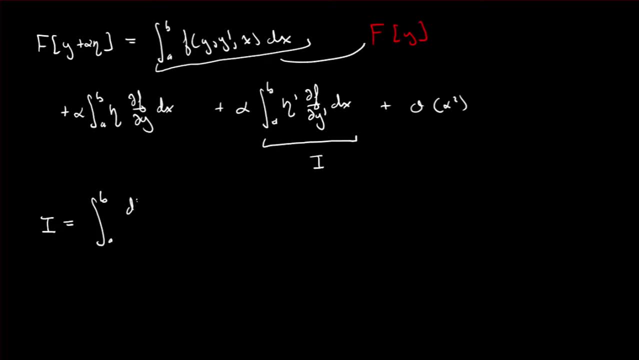 to write that as d eta, as d eta, dx times, d, f, dy, prime, dx. And now you can probably see how we're going to simplify this, because this is a derivative with respect to x times, something that's not differentiated with respect to x and the. 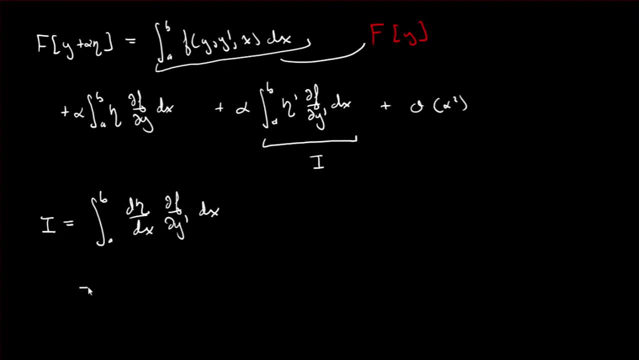 integral is with respect to x. so you can probably see that to simplify this we are completely within our rights to use the integration by parts technique to simplify this. So we write: this is eta of x, Times, d, f, dy, prime, and this has got to be evaluated from a to b. so we peel the derivative. 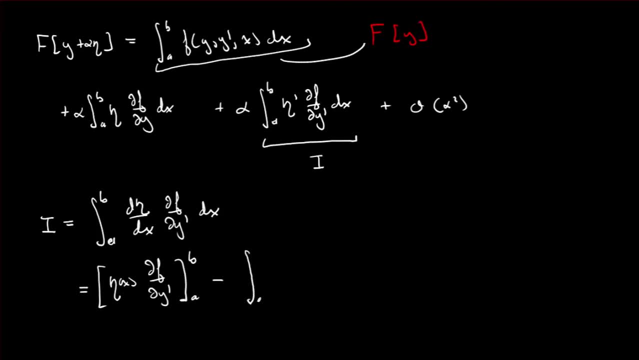 of eta, then we subtract off the integral from a to b of, and now we take the integral of eta and we stick it on to d f, dy prime. So that's the derivative with respect to x of d f, dy prime, dx. So what we've done is: 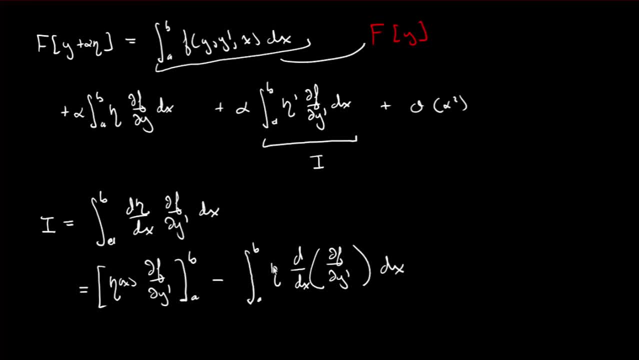 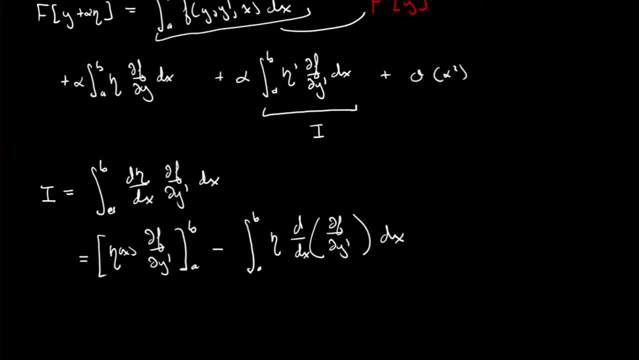 evaluated this at the boundaries and we've moved the derivative off eta and onto df, dy, prime, and that's integration by parts. We can make it yet simpler because, look at this, Remember from before, we were quite careful to define eta. We were quite careful to define eta so that eta of a 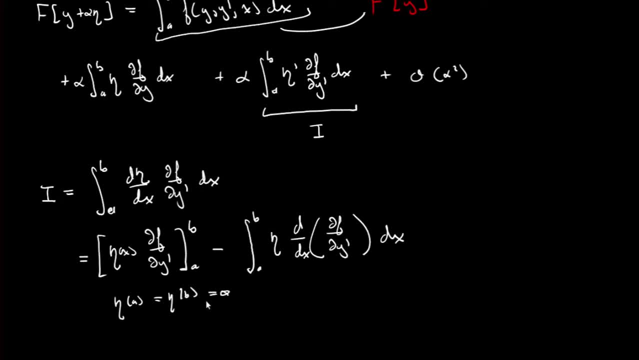 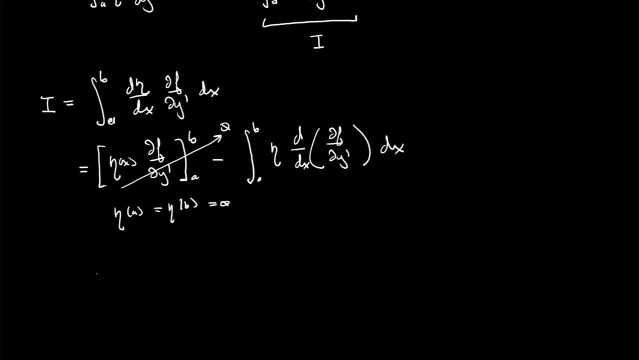 is equal to eta, of b is equal to zero, But eta's in this term. It's in this term that we're evaluating at the boundaries, but it vanishes at the boundaries. Therefore, this whole term just vanishes. We can ignore it and that's just a consequence of us choosing eta to be. 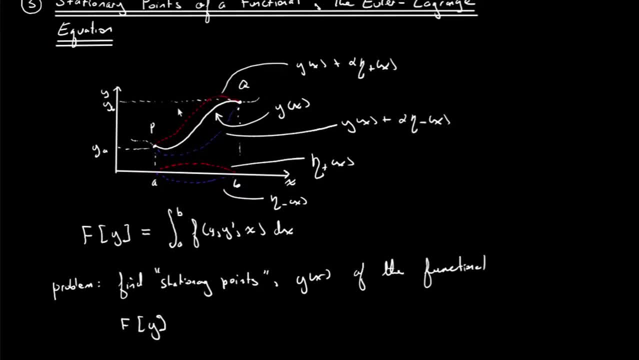 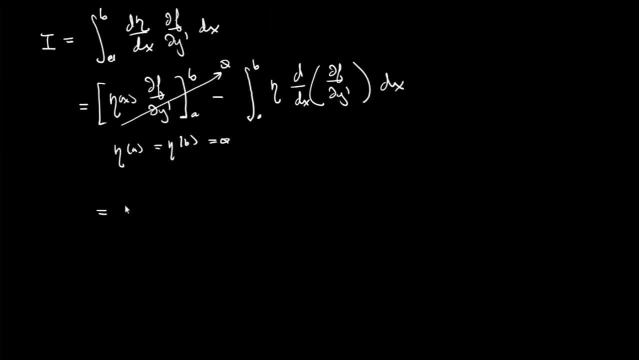 an honest to goodness variation, so that we always land on the endpoints, no matter how we vary it. And well, we have this left over, the integral from a to b of eta, d, dx, of df, dy, prime, and this is integrated with respect to x. And now, well, we can just go back. 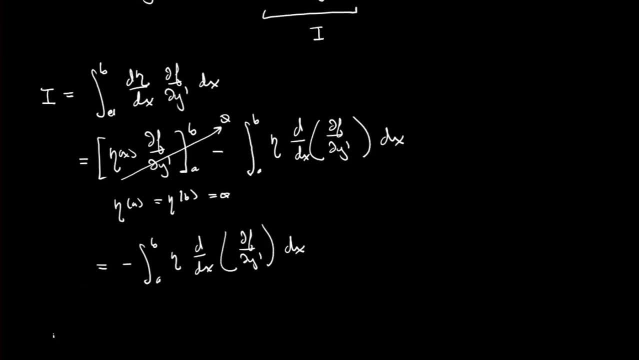 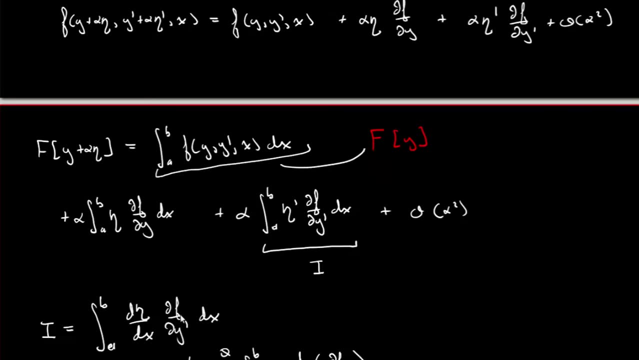 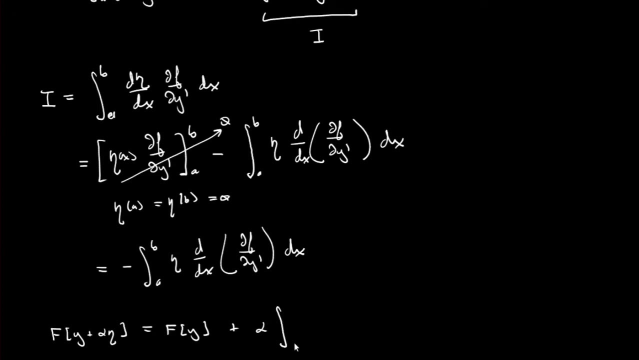 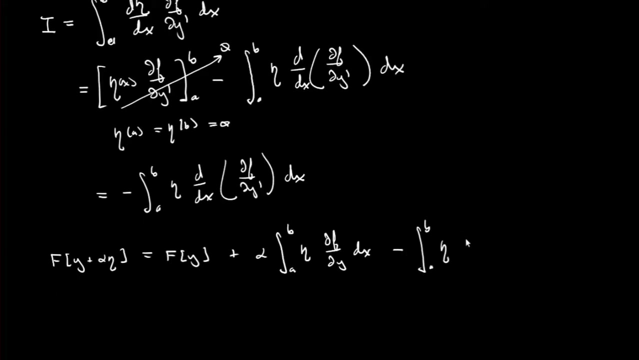 to our functional right. So our functional evaluated as our displaced point, f of y plus alpha, eta, That's just going to be equal to well, that's f of y plus alpha. integral from a to b, eta, df, dy, dx. But now our newest term, integral from a to b of eta, And this is the derivative. 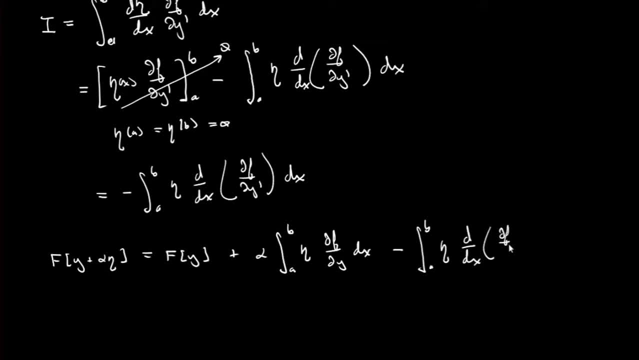 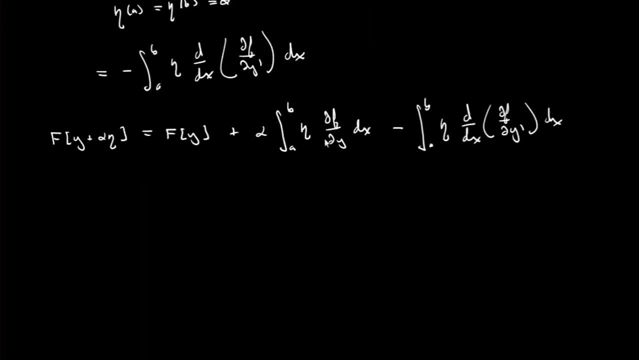 with respect to x, of df, dy, prime, and that's with respect to x as well. And we see we can put these together because- notice- there's a common factor of eta in these two integrals brands. So we can really put them together in quite a nice way. So, of course, please, 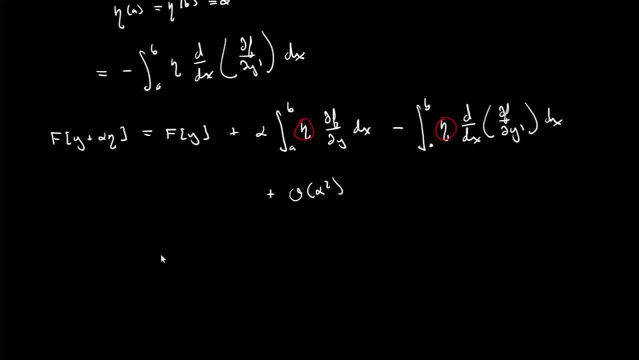 forgive me for forgetting our big O of alpha squared, And this then becomes well f of y plus alpha, And of course I've got my alpha here as well. integral from a to b of eta, And this is eta as a function of x. Now, this is times df, dy, And that came from here We're. 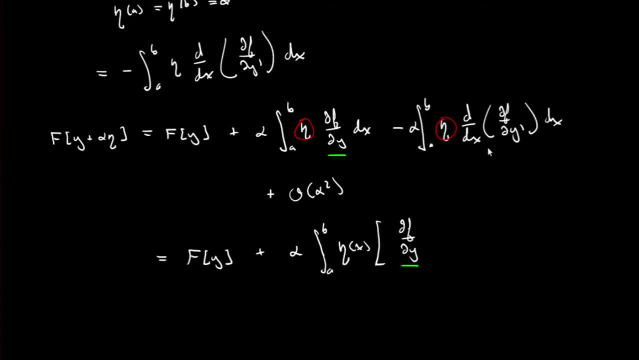 just collecting what's in the other bracket, what's in the other, integrand over here We're collecting this And that's going to come as a minus because we're collecting a minus sign times d, dx, df, d, y, prime- And that's to be integrated with respect to x And of course that came from. 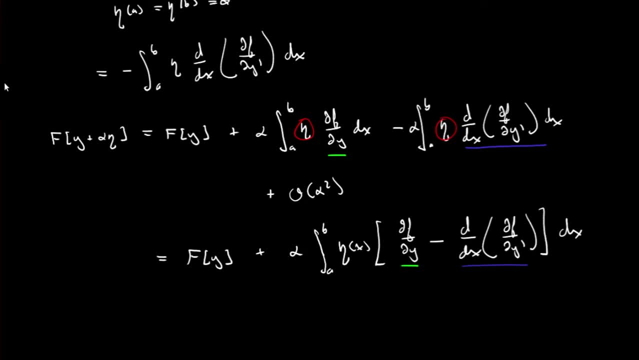 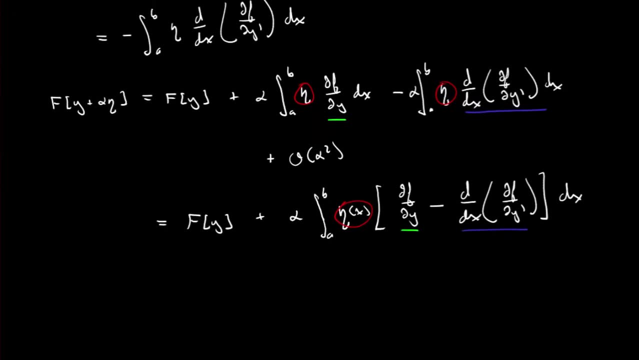 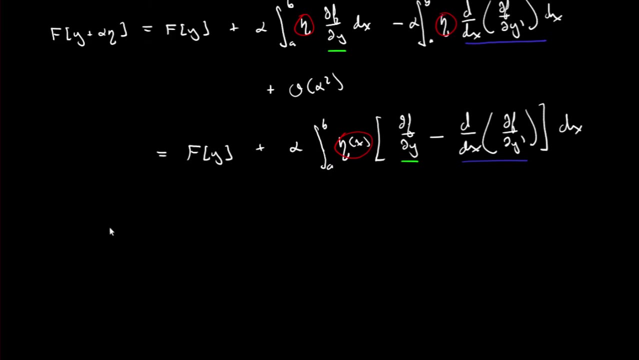 here, That's that term there, And of course the eta is just the same eta from over there. So we've collected them. Now this is the payload. This is where we kind of get the result of all our hard work. We just move the f of y over to the other side and we 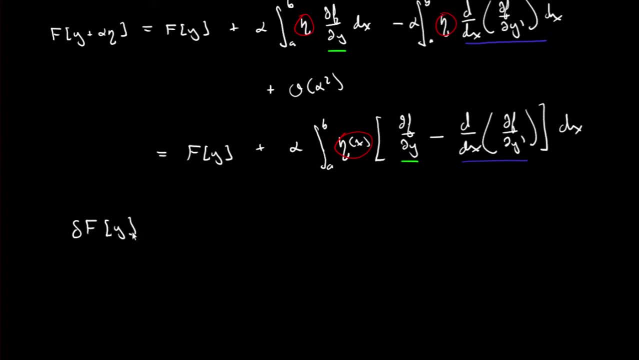 have delta f And then we've got beta. f of y is just f of y plus alpha eta minus f of y And that's just equal to. of course I forgot my plus o of alpha squared here. That's going to be equal to just alpha integral from a to b of eta of x times our funny, funny expressions. I'm sorry, I just can't remember. Seriously, the hice of b to alpha is just f of y, d, d minus dx, that's just equal. of course I forgot my plus o of alpha squared here. that's going to be equal to just alpha integral. from a to b of eta of x times our funny, funny expression. 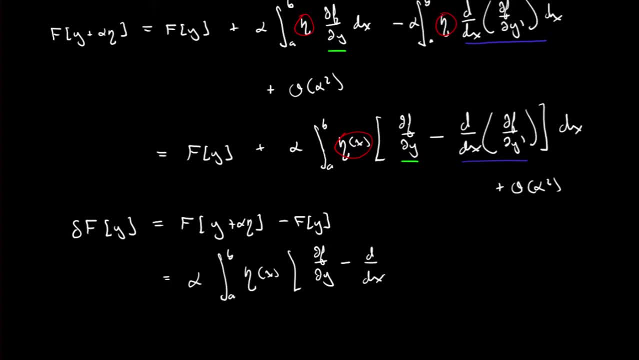 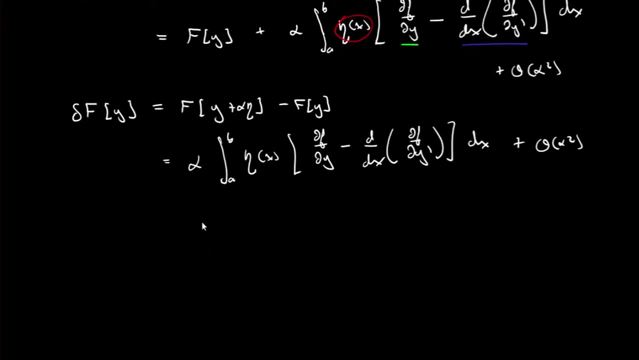 here df, dy minus d, dx, the derivative with respect to x of the partial derivative of f with respect to y, prime, all integrated with respect to x, plus higher order terms in alpha. Now this alpha, remember, it's small but not zero. So small but critical. 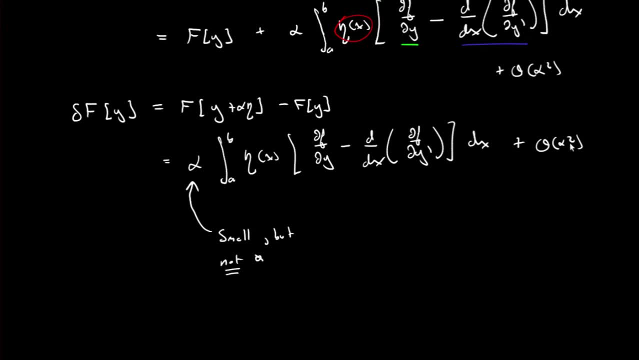 is basically not zero And we choose alpha to be small enough for higher order terms to be negligible. Therefore, the only way for this to vanish is if, for all, x this to this integrand vanishes right, Because, remember, eta is arbitrary. eta is completely arbitrary. 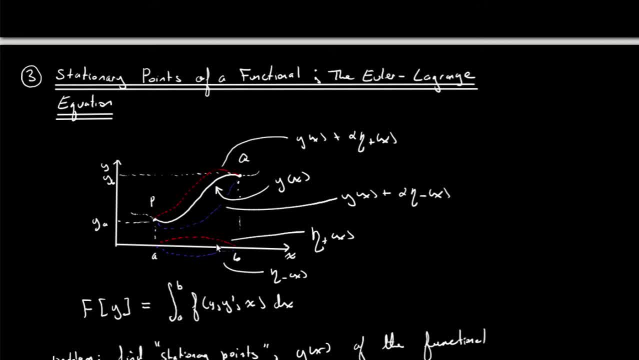 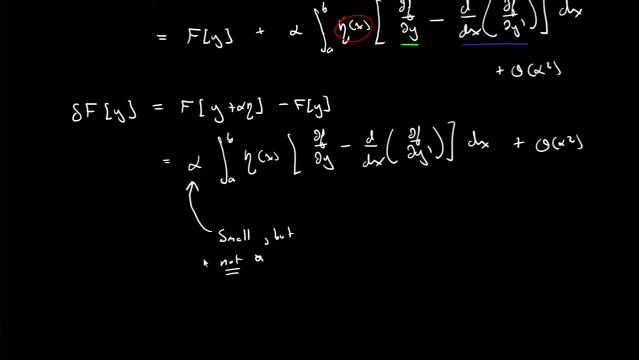 just so long as it vanishes at the end point. If it vanishes at the end point, it's a good variation. We can drag its magnitude down a certain small as we want, because it's multiplying that tiny, tiny alpha there, right, But eta. 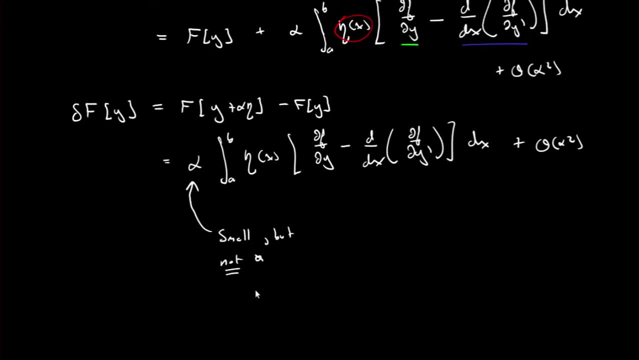 is, in principle, arbitrary just so long as it satisfies the boundary conditions. So because eta is arbitrary, we, you know it doesn't have to be zero, right We to guarantee that this is always zero. we would need for this to vanish. we need this to vanish And that's. 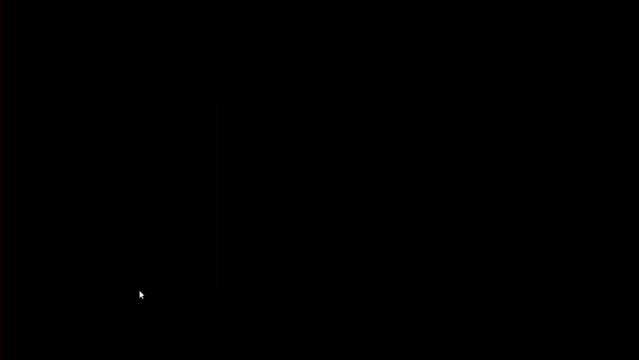 our condition. So this is our condition, which we're going to write here. We're going to write bright and shiny on a new page as the partial derivative of f with respect to y minus the derivative with respect to x of the partial derivative of f with respect. 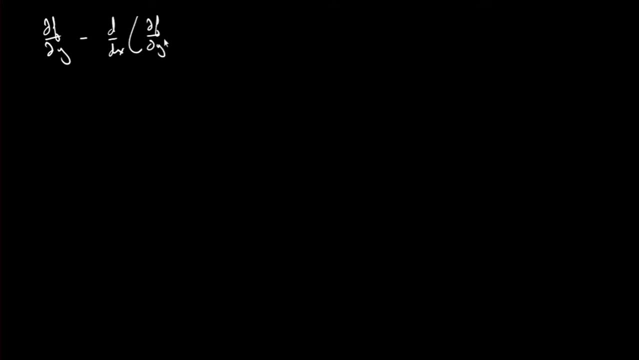 to y prime. That's got to vanish. And this is a condition. that's equivalent to the statement that y makes f of y. So if y satisfies this differential equation, we say that y makes the functional capital F of y stationary. And what's also worth pointing out is this: this has a name, It's a differential. 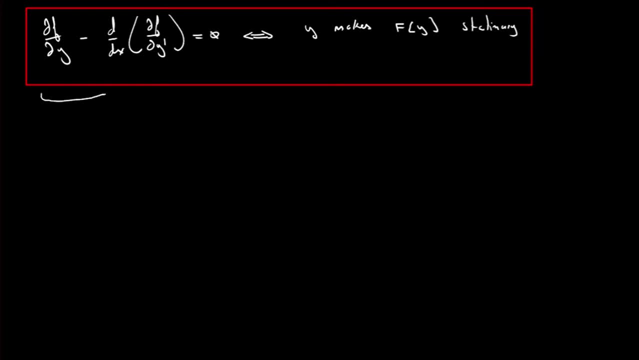 equation. It's a differential equation And when we solve it we get y as a function of x And it's called the Euler throw-in Lagrange equation. So this is the Euler-Lagrange differential equation. It's worth also pointing. 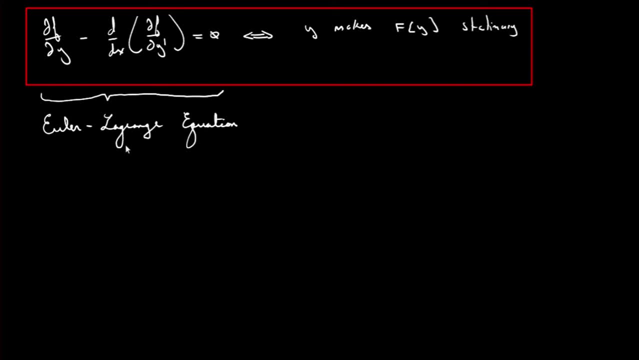 out that, remember, for the 1D case this object was just the derivative with respect to x of our function And in the 2D case it was another kind of derivative: It was the gradient, which was a vector-valued function And in higher dimensions in the general case, in 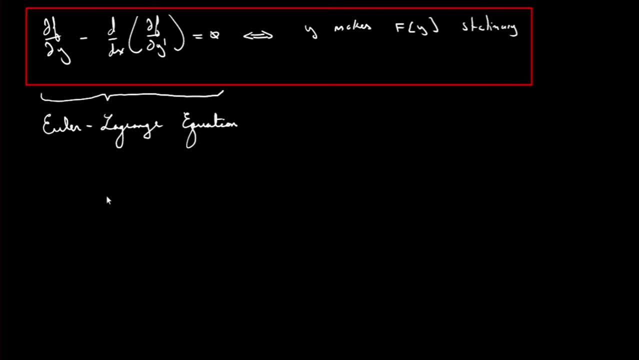 n dimensions, we got an n-dimensional gradient. Well, really, what that tells us is that we should think of this object appearing on the left-hand side of the Euler-Lagrange equation as a kind of derivative. And we do, We give it a name, We call it the functional derivative. 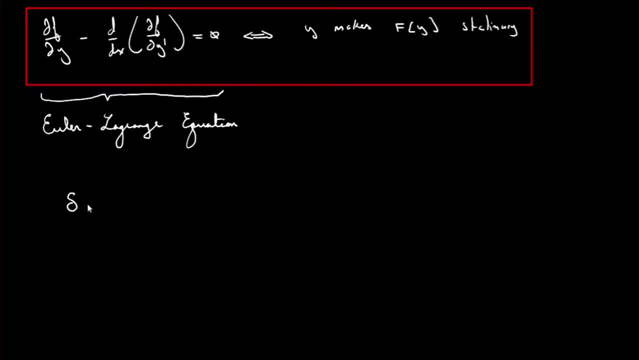 So we write that the functional derivative df of y with respect to y of x, We call that the partial derivative of f with respect to y, minus the total derivative of f with respect to y prime. So essentially the Euler-Lagrange. 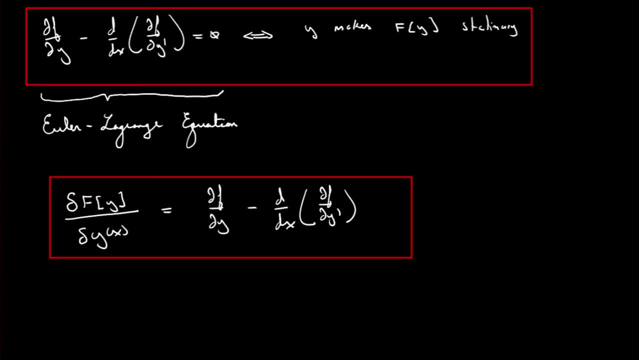 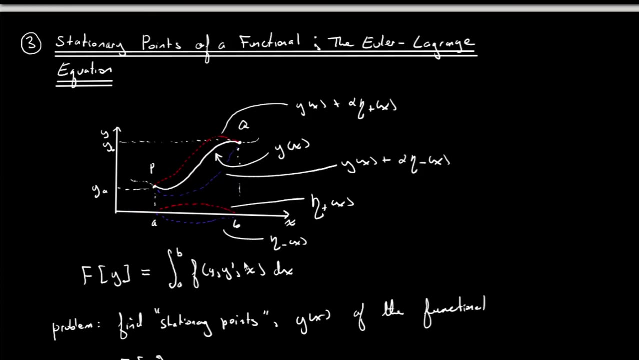 equation is just the statement that this functional derivative vanishes. And now this is the payoff. Euler-Grange equations. we can analyze any problem whatsoever where we want to make some functional stationary. So if we want to find what y of x makes some functional stationary, 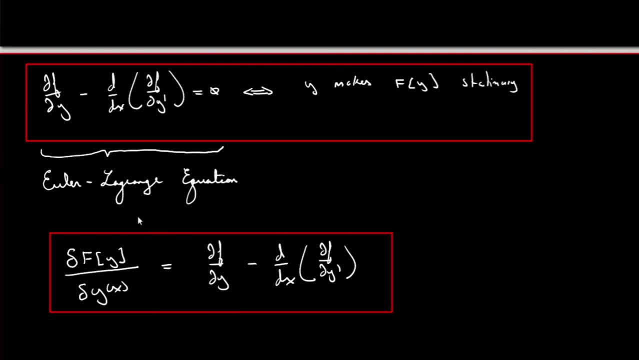 we just have to solve this differential equation, And next time we're going to go back to our example right from the beginning that we used to motivate the calculus of variations. We're going to bring this tool to bear on the problem of finding the function that minimizes the 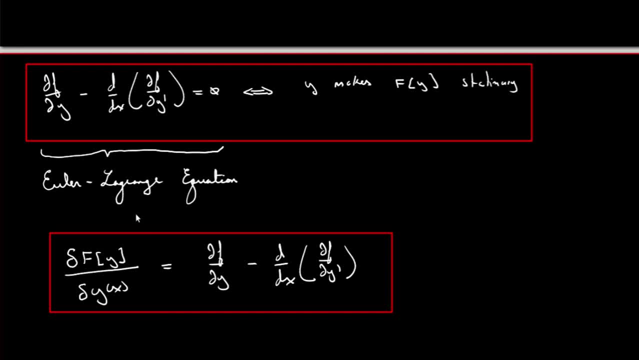 traversal distance between a point P and a point Q.